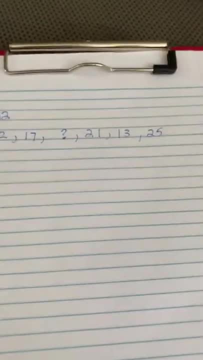 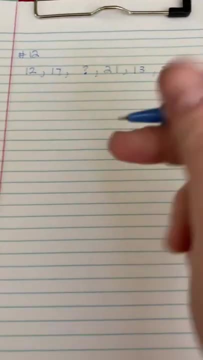 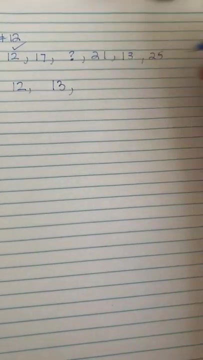 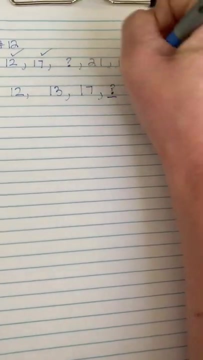 Okay, so if we're looking for the median, we're looking for the number that would fall in the middle of our data set, So the first thing we need to do, though, is put them in order least to greatest. So our smallest would be 12,, then 13,, then 17,, then our question mark- we don't know what that value is yet- then 21 and 25.. 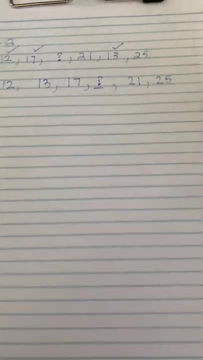 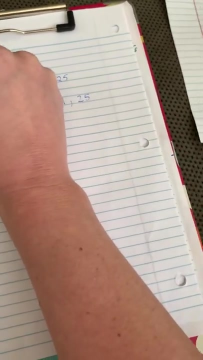 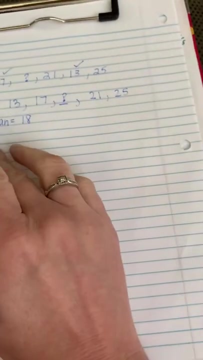 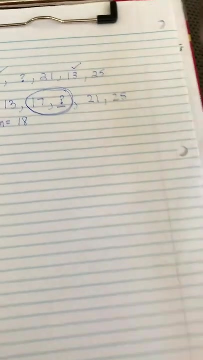 So this is where it gets confusing. So our median has to be 18.. That's what it told us, And number 12.. So when we have an even number- 1,, 2,, 3,, 4,, 5,, 6,- our middle would be between our two numbers here in the middle. 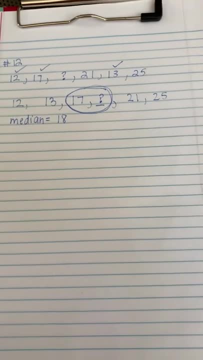 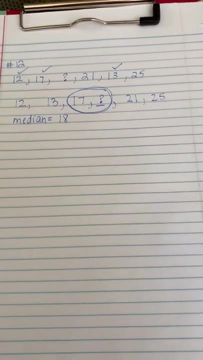 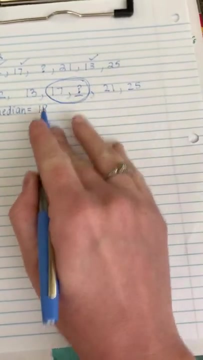 An odd data set with an odd number is very easy Because it's one number in the middle of our data set. Here we have 2, and it says our median has to be 19.. So that means or 18,. I'm sorry, that means the average of these two is going to be 18.. 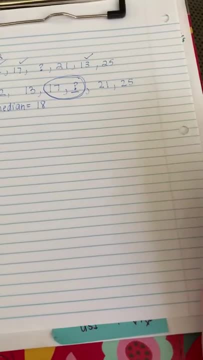 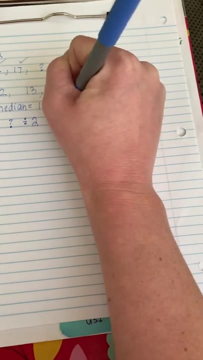 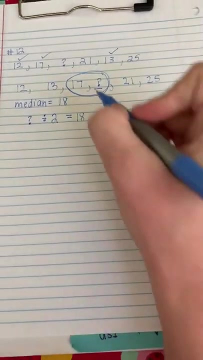 So what you can do is you can think what number divided by 2 equals 18.. Okay, So what you can do is you would add them together and divide by 2.. Let's go So when we have a missing number, you have to go backwards. 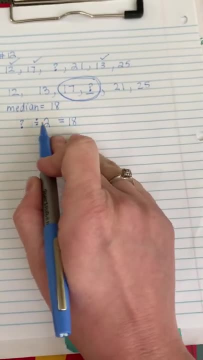 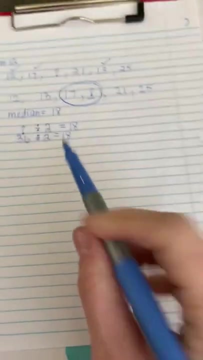 Okay, So what number then? divide by 2 equals 18?? Well, 18 times 2 is 36,. so 36 divided by 2 equals 18.. Okay, So the sum of these two numbers has to equal 36, because when we divide it by 2, it has to be 18.. 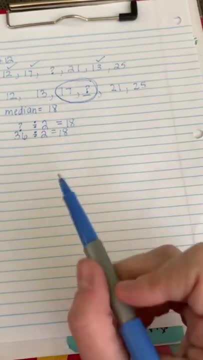 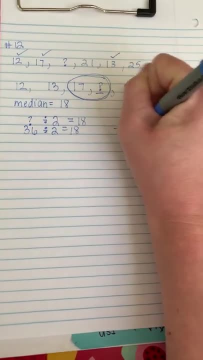 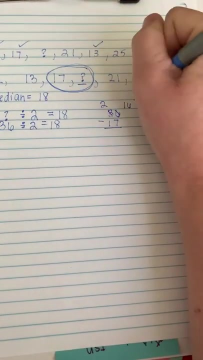 Well, to figure that out, we can find the difference by subtracting. Okay, so 36 minus 17,. we've got to make this a 16 and make this 3 a 2.. 16 minus 7 is 9,. 2 minus 1 is 1..